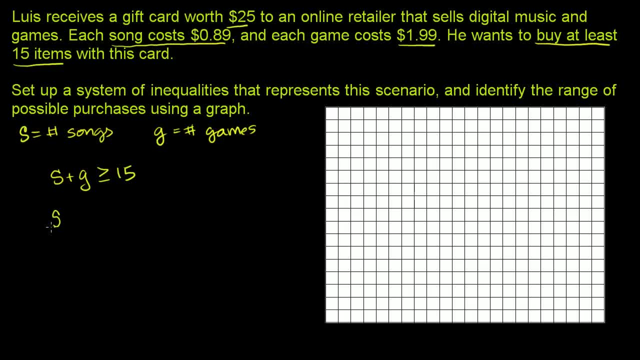 So the amount that he spends on songs are going to be the number of songs he buys times the cost per song, times $0.89.. I'll say 0.89 times s. That's how much he buys, That's how much he spends on songs, plus the cost per game. 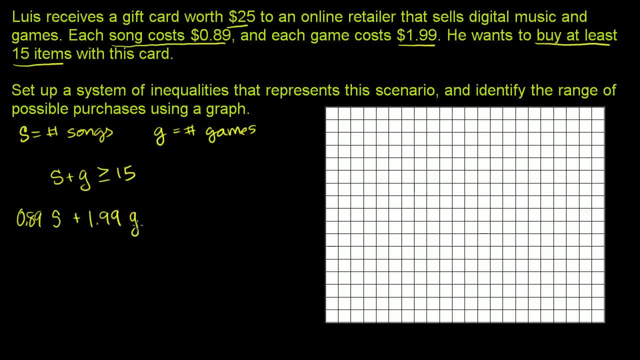 which is $1.99, times the number of games. This is going to be the total amount that he spends, And that has to be less than or equal to 25.. Now, if we want to graph these, we first kind of have to. 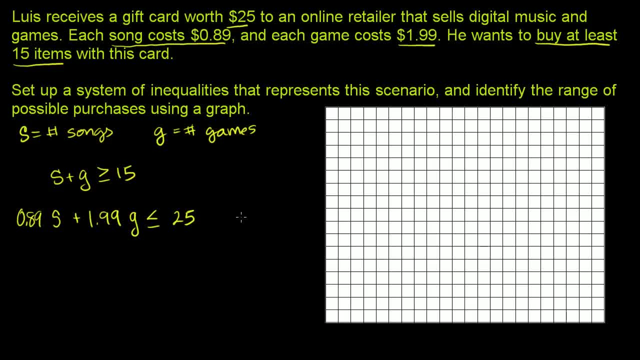 define the axes. So let me do that right here. And we only care about the first quadrant because we only care about positive values for the number of songs and the number of games. We don't talk about scenarios where he'd be buying a lot of. 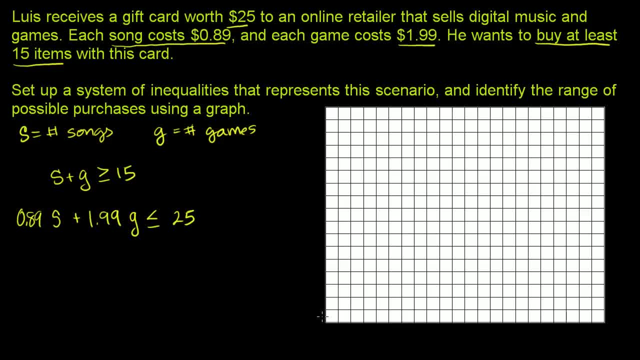 games. He buys a negative number of songs or games. So this is going to be just the positive quadrant. right here Let me draw the axes. So let's make the vertical axis that I'm drawing right here. Let's make that the vertical axis. 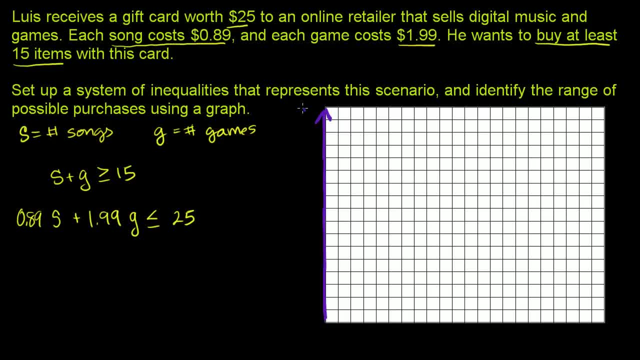 And let's call that the song axis. So that's the number of songs he buys. Let me make sure you can see that That is the song axis, And then let's make this horizontal. That's going to be the number of games he buys. 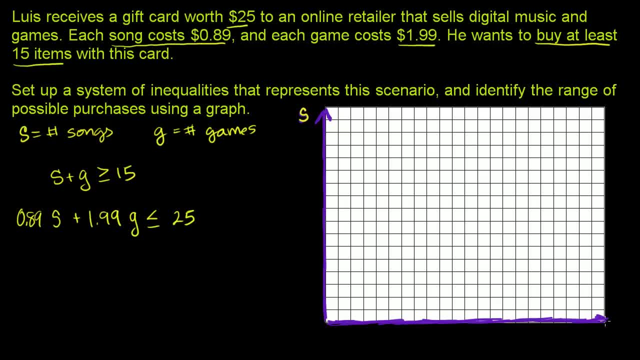 Just bold it in And just to make sure that we can fit on this page, because I have a feeling we're going to get to reasonably large numbers, let's make each of these boxes equal to 2.. So this would be 4,, 8,, 12,, 16,, 20, so on and so forth. 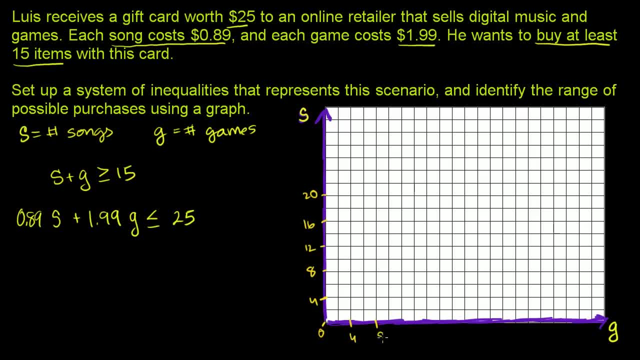 would be 4,. this obviously would be 0,, 4,, 8,, 12,, 16,, 20, and so on. So let's see if we can graph these two constraints. Well, this first constraint, s plus g, is going to be: 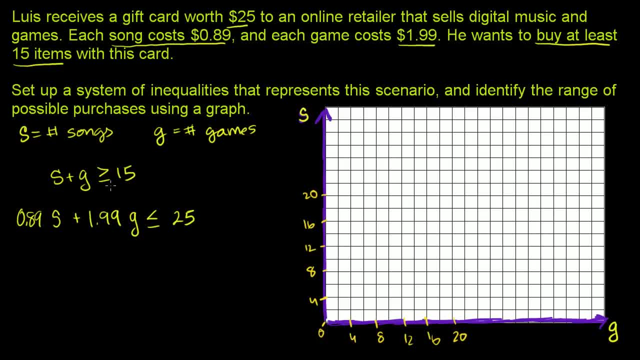 greater than or equal to 15.. The easiest way to think about this, or the easiest way to graph this, is to really think about the intercepts. If g is 0, what is s Well s plus 0 has to be greater than or equal to 15.. 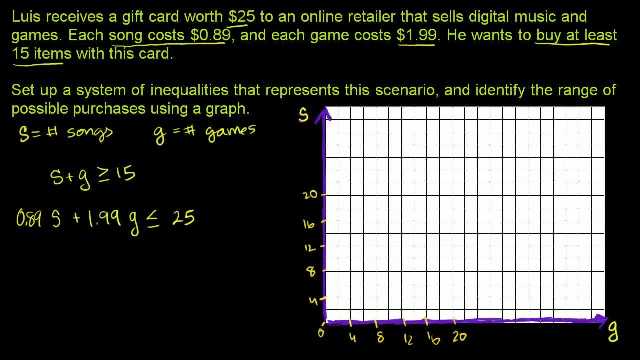 So if g is 0, s is going to be greater than or equal to 15.. Let me put it this way. So, if I'm going to graph this one right here, if g is 0, s is greater than or equal to 15.. 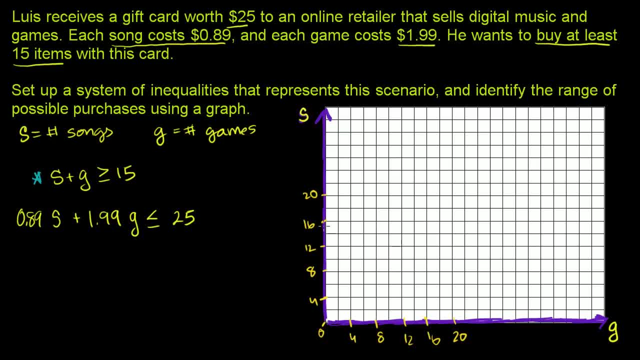 So g is 0, s, 15 is 12,, 14,, 15 is right over there, and s is going to be all of the values equivalent to that or greater than for g equal to 0.. If s is equal to 0, g is greater than or equal to 15.. 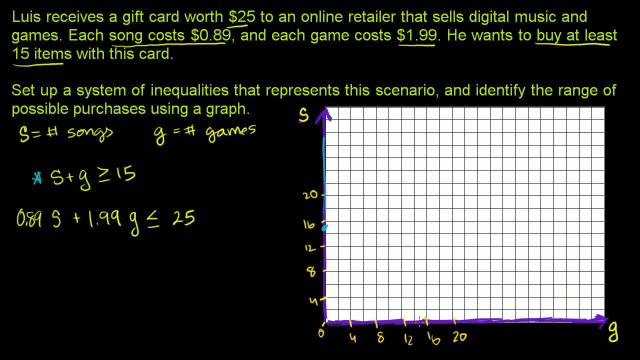 So if s is equal to 0,, g is greater than or equal to 15.. So g is greater than or equal to 15.. So the boundary line s plus g is equal to 15.. We would just have to connect these two dots. 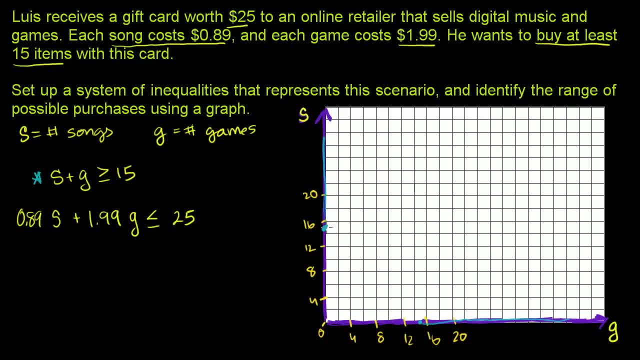 Let me try my best to connect these dots, So it would look something like this: This is always the hardest part. Let me see how well I can connect these two dots. Nope, I should get a line tool for this. So that's pretty good. 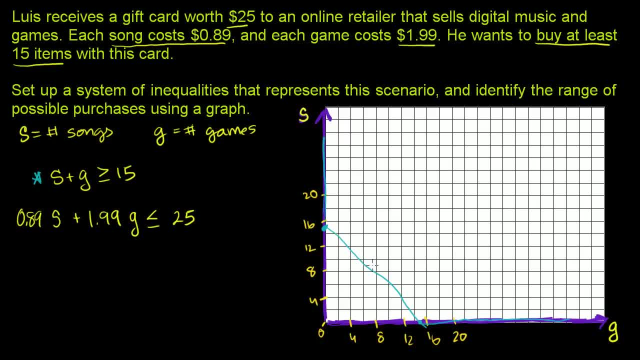 So that's the line: s plus g is equal to 15.. And when we talk about the values greater than 15, we're going to go above the line. You saw that when g is equal to 0, s is greater than or equal. 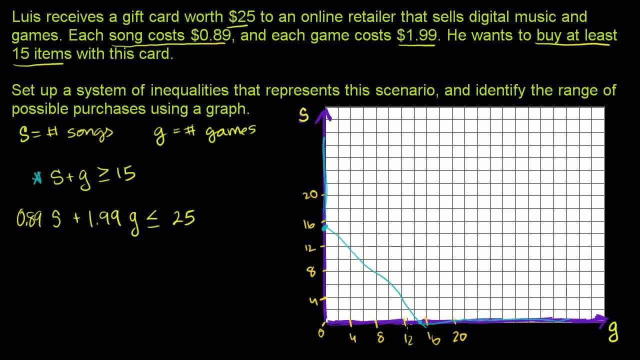 to 15.. It's all of these values up here, And when s was 0,, g was greater than or equal to 15.. So this constraint, This constraint right here is all of this area, satisfies this, All of this area. if you pick any coordinate here, it. 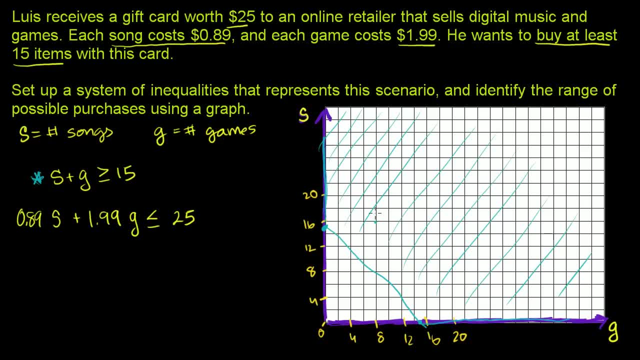 represents- and really you should think about the integer coordinates, because we're not going to buy parts of games. But if you think about all of the integer coordinates here, they represent combinations of s and g where you're buying at least 15 games. 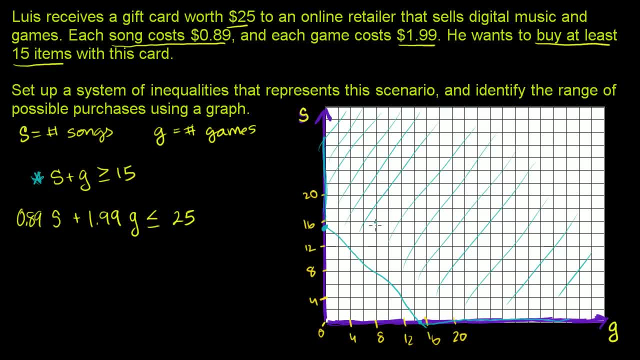 For example, here you're buying 8 games and 16 songs. That's 24.. So you're definitely meeting the first constraint. Now the second constraint: 0.89.. s plus 1.99 g is less than or equal to 25.. 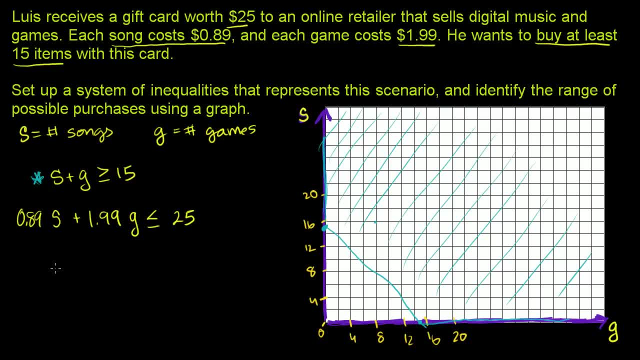 This is a starting point. Let's just draw the line. Let's draw the line: 0.89 s plus 1.99 is equal to 25.. And then we could think about what region the less than would represent, or 1.99 g. 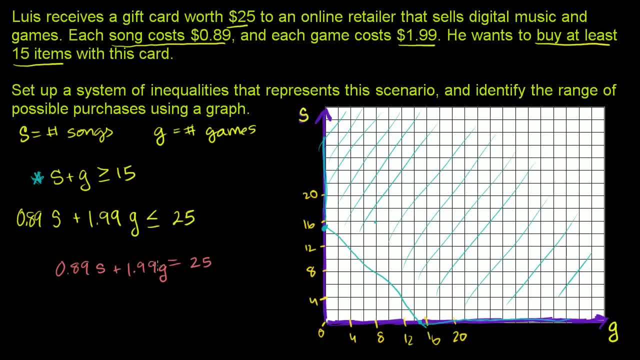 And the easiest way to do this. once again, we could do slope y-intercept and all of that type of thing, But the easiest way is to just find the s and the g intercepts. So if s is equal to 0.99.. 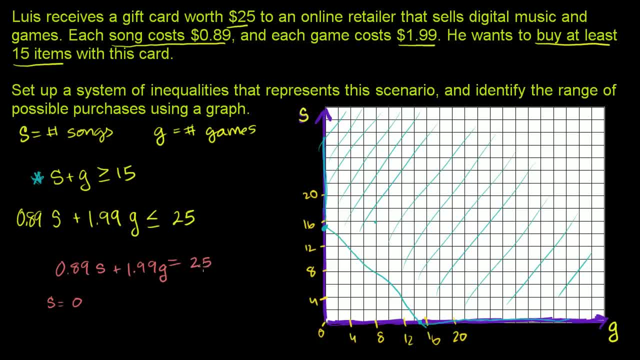 If s is equal to 0,, then we have 1.99. g is equal to 25.. So s is equal to 0, then we have 1.99. g is equal to 25.. Or g is equal to. let's get a calculator out for this. 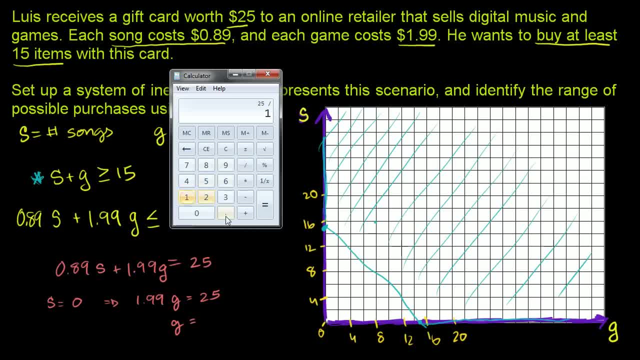 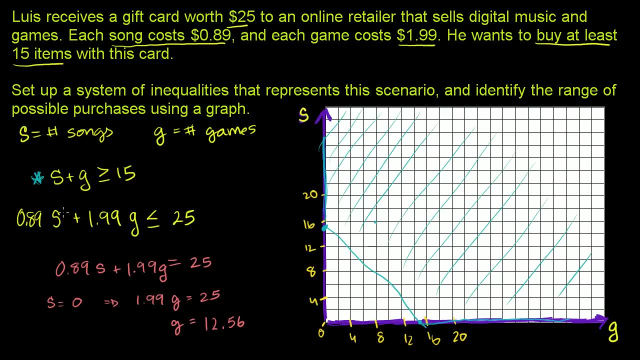 So if we take 25 divided by 1.99, it is 12.56.. g is equal to 12.56.. Let me get it 12.56.. And then, if so, when s is 0,, let me plot this. 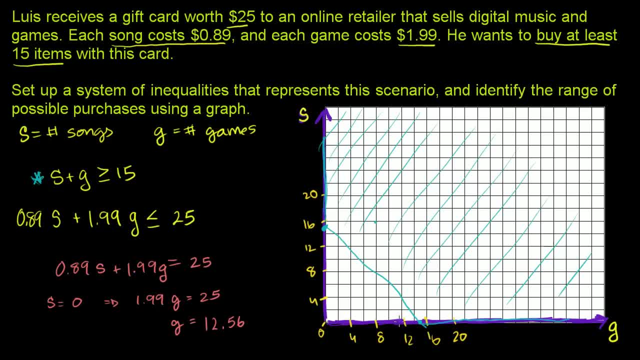 When s is 0, g is 12.56.. This is 12.. This is 14.. 12.56 is going to be right there, A little bit more than 12.. That's that value there, And then let's do the same thing if g is 0. 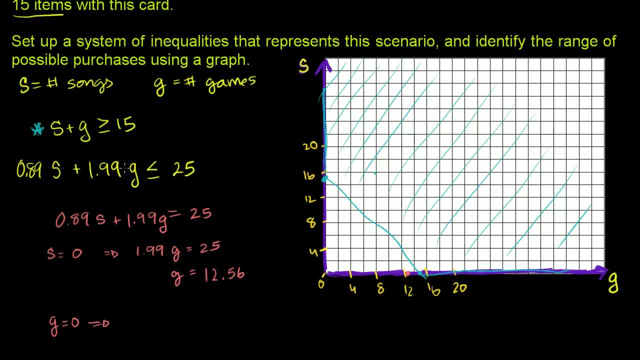 So if g is equal to 0,, then we have, so this term goes away. we have 0.89 s if we use just the equality here, the equation. So if we have g is equal to 0, g is equal to 25 or s is equal. 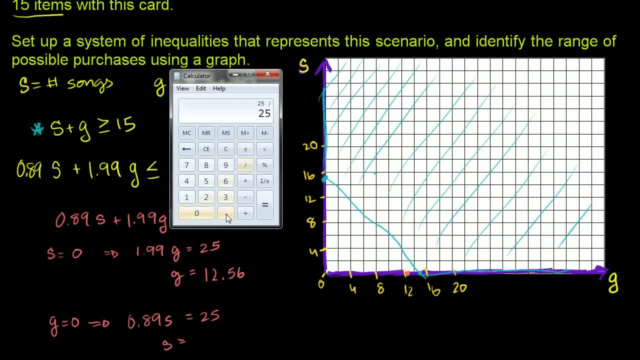 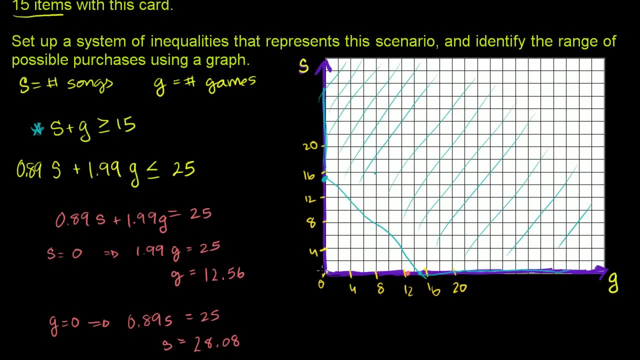 to get the calculator out again. So if we take 25 divided by 0.89, we get it's equal to 28.08.. Just a little over 28,, so 28.08.. So that is, g is 0, s is 28.. So that is 2, 4.. 24.68.. A little over 28.. So that is: g is 0, s is 28.. So that is 2, 4. 24.68.. So that is, g is 0, s is 28.. So that is 2, 4.24.68, a little over 28.. 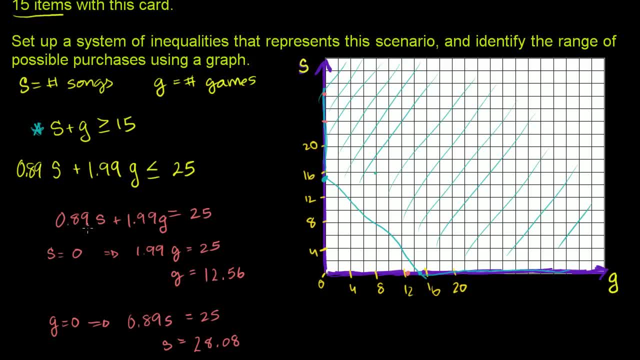 So it's right over there. So this line- 0.89s plus 199g is equal to 25, is going to go from this coordinate, which is 0, 28,. so that point right there, all the way down to the point 12.560.. 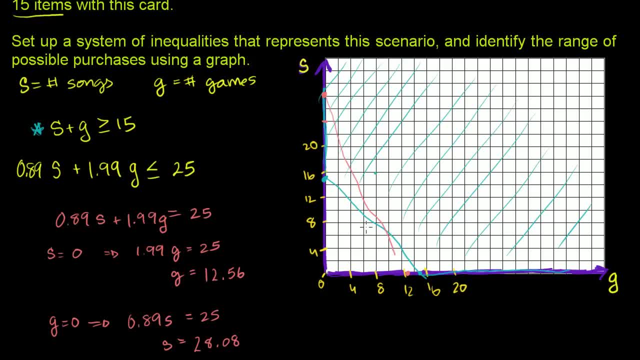 So let me see if I can draw that One more attempt. Maybe if I start from the bottom it'll be easier. That was a better attempt. Let me bold that in a little bit so you can make sure you can see it. 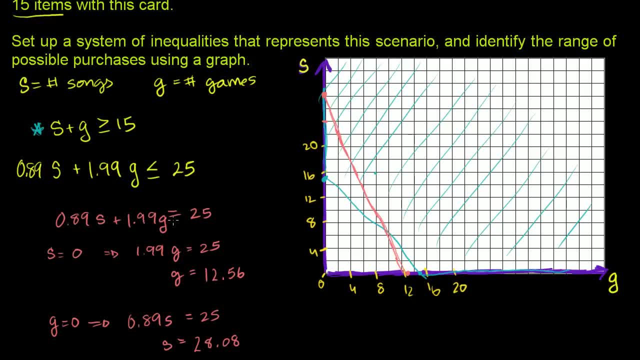 So that line represents this right over here. Now, if we're talking about the less than area, what will that imply? So, if we think about it, when g is equal to 0, 0.89s is less than 25.. 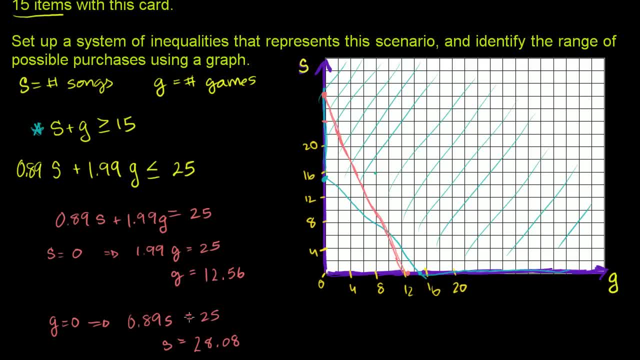 So when g is equal to 0, if we really wanted the less than there, we could think of it this way: It's less than, instead of just doing less than less than Or equal to. So s is less than 28.08.. 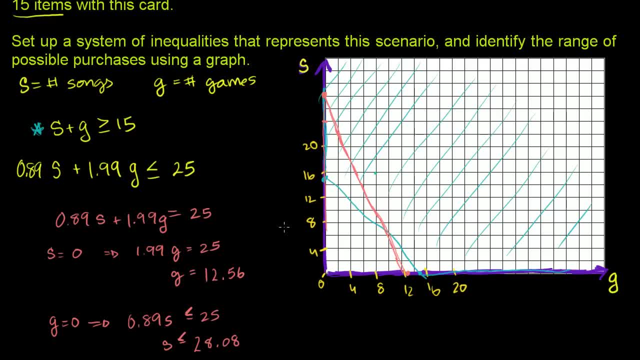 So it'll be the region below. So if we think s is 0,, if we use this original equation, 199g will be less than or equal to. I used this just to plot the graph, but if we actually care about the actual inequality we get 199g is less than 25.. 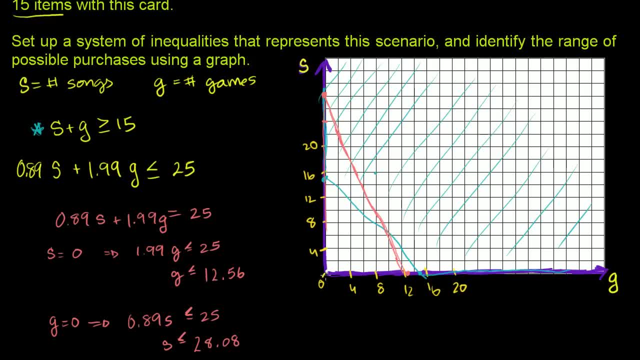 g would be less than or equal to 12.56.. So when s is equal to 0. g is less than 12.56.. So the area that satisfies this second constraint is everything below this graph. Now we want the region that satisfies both constraints. 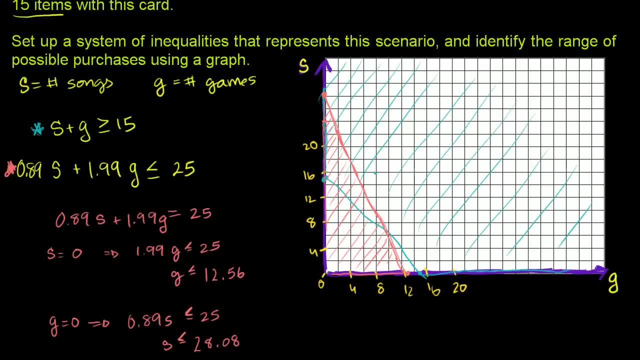 So it's going to be the overlap of the regions that satisfy one of the two. So the overlap is going to be this region right here below the orange graph and above the blue graph, including the two, including both of them. So if you pick any combination, so if he buys, 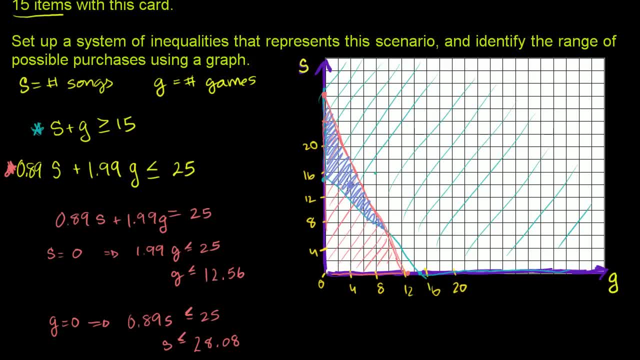 four games and 14 songs, that would work. Or if we bought two games and 16 songs, that would work. So you can kind of get the idea. Anything in that region and he can only buy integer values would satisfy both constraints.